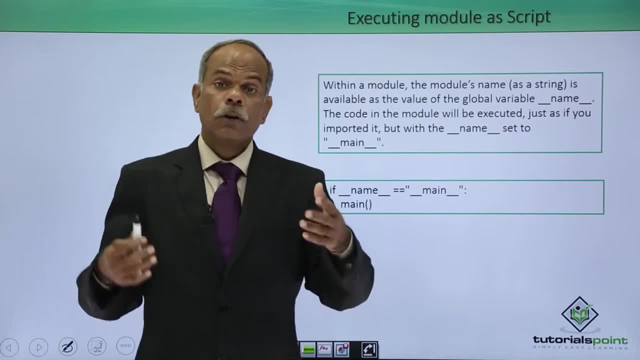 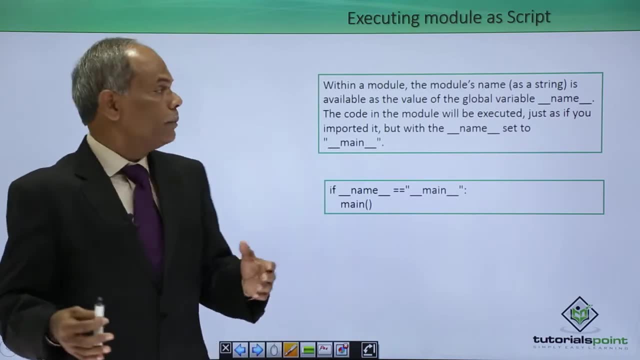 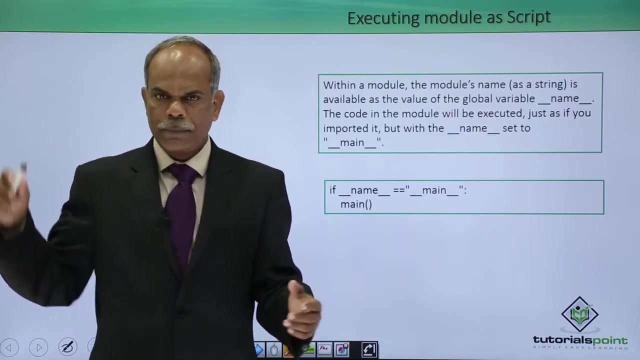 another script which is a module, But the module itself can be used as a starting point of your execution. How is it done? This is possible because the module's name. you save the name, the module by certain name- module1.py. So module1 becomes the name of the module. 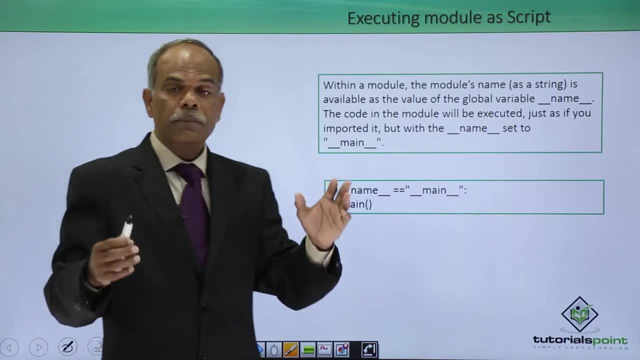 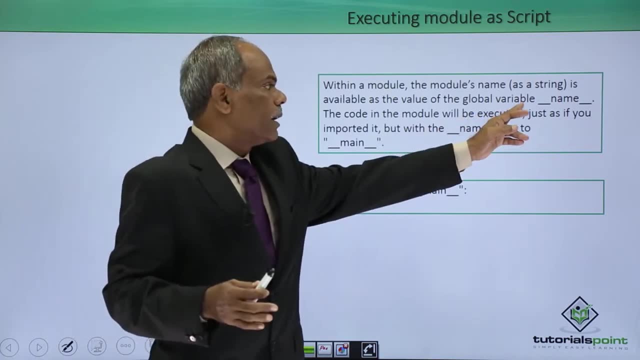 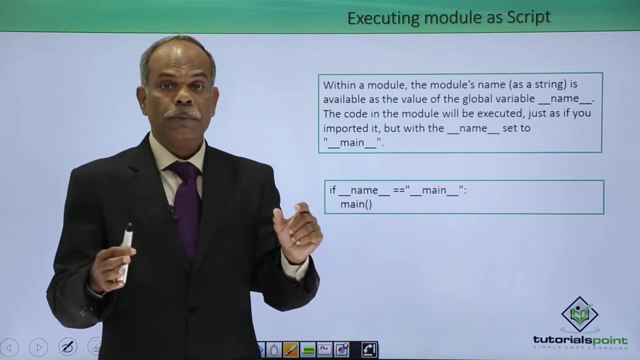 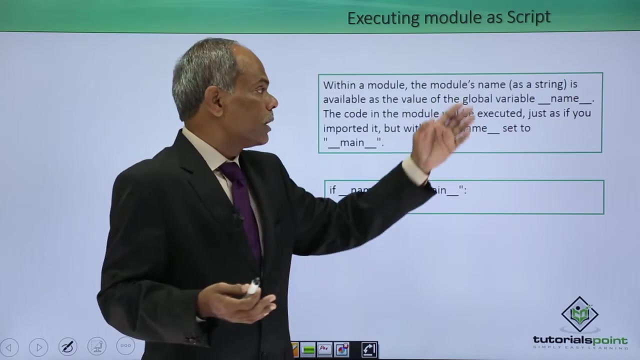 Now that module's name, which is a string, is available as a value to a defined global variable, called as double underscore name. double underscore- So this is a spatial syntax used to some specially reserved function names which are called as magic methods. This is a magic method, So double underscore name under double underscore. this is a spatial 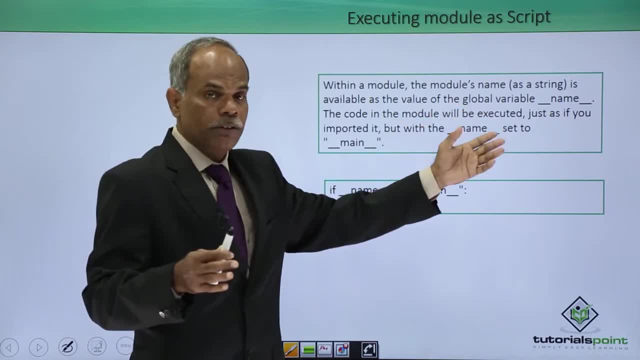 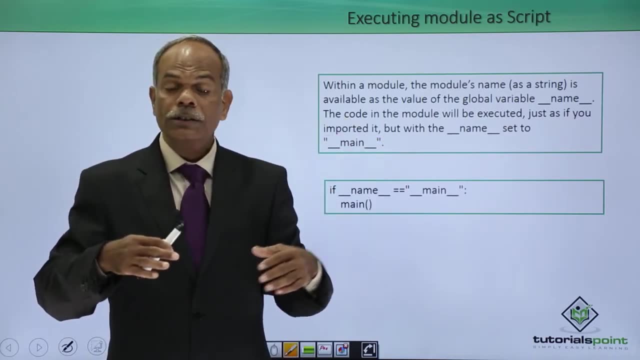 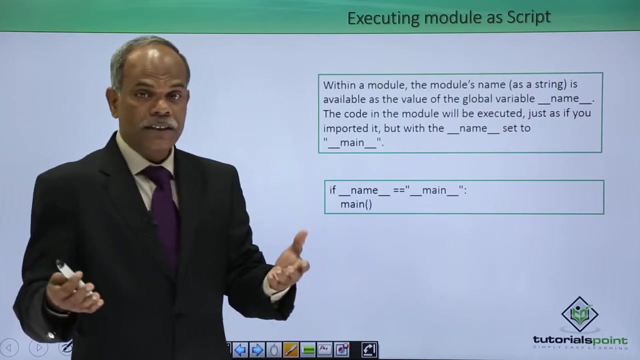 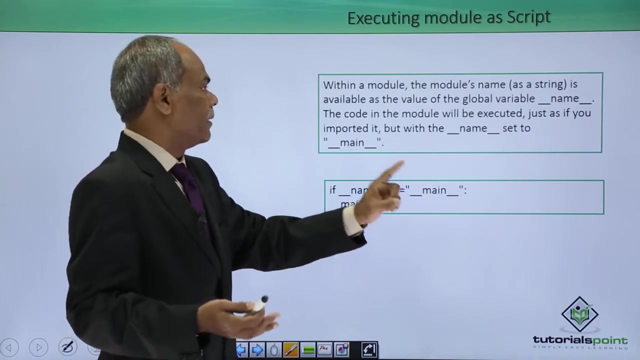 name, which is rather a global variable and which stores the name of the current module, The which module is being executed, which script is being executed, its name is stored in this variable. Obviously, when the script is being used, rather executed, that name of the script is main. 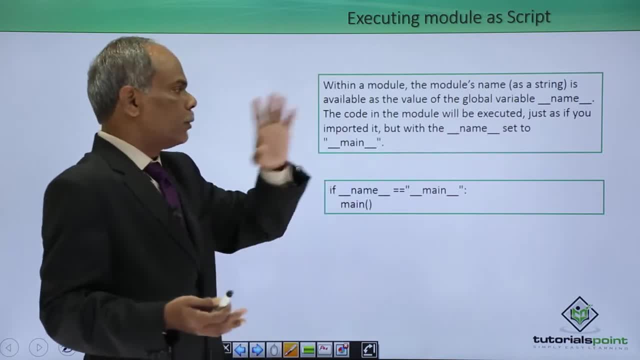 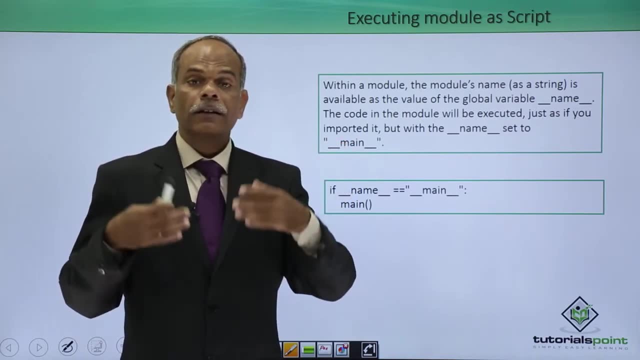 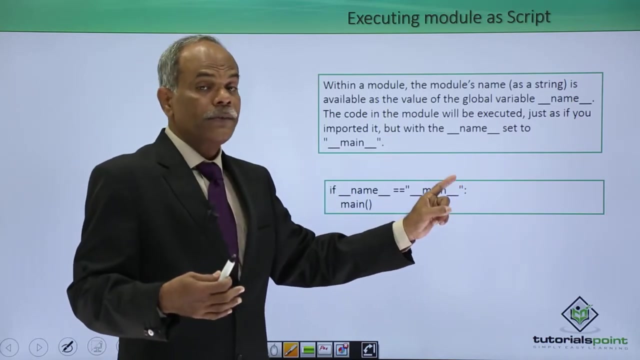 The code in the module will be executed just as if you have imported it, but with the name set to main. So what does it mean? When a particular script is executed, the script that is executed, its name is main. If the module is imported from somewhere, its name is not main. 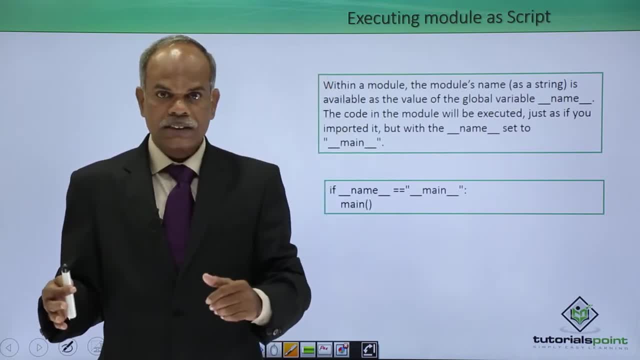 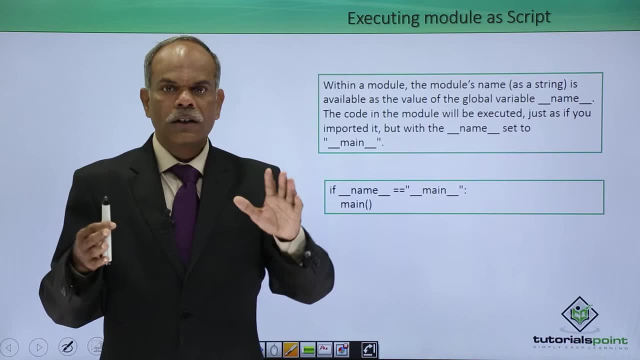 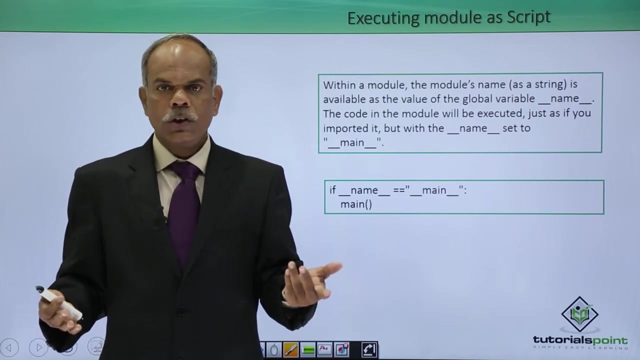 So if I have a module in which there are certain functions, and I will test it when I try to run that program- If the module contains only functions and there is no call to the function, then obviously nothing happens. Nothing will run. What you have to do. 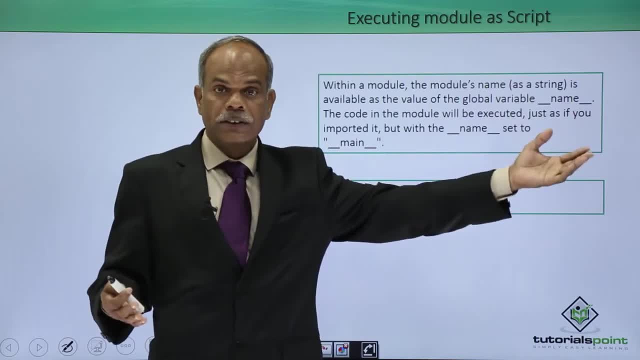 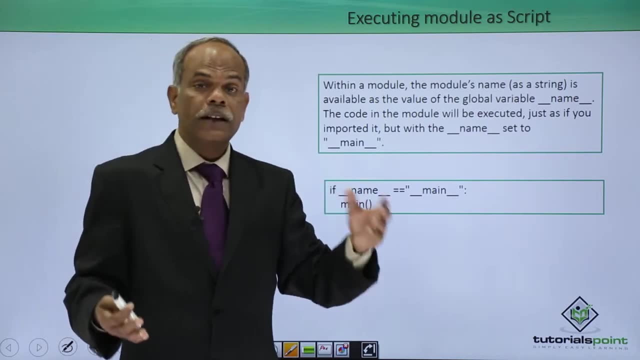 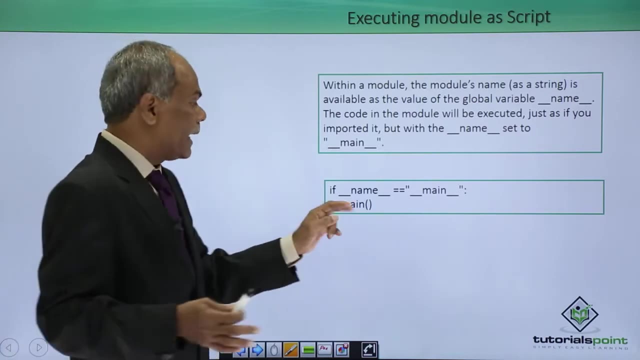 You have to run those functions from some other functions or from other script by importing it. But if I want to run the functions which are defined in the module itself, what do I have to do? I have to check whether this is the current script that is being executed and that I can. do by testing it. If name equal to main, If I have a, If I have executing that script itself, its name will become main. This condition will be true. Then if there is a main function called as main in the script, that will be executed. 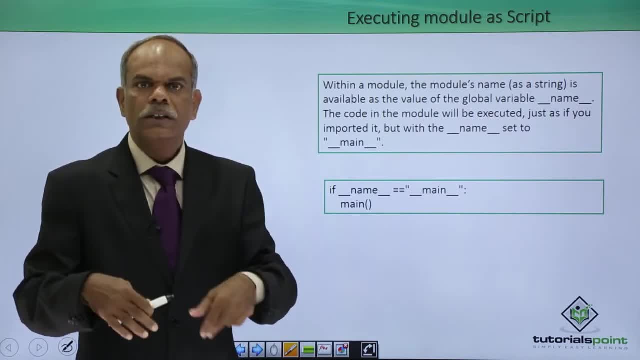 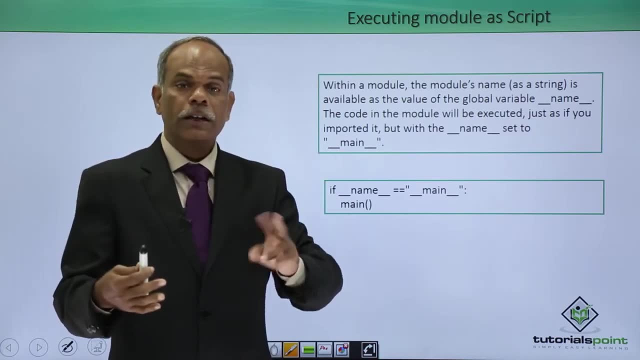 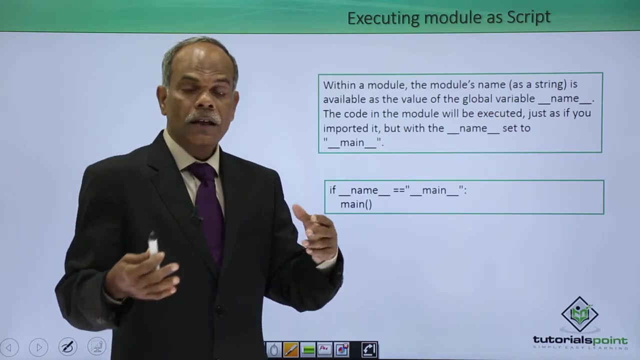 So either way, the script can be incorporated into other script by using the import, or you can execute that script itself. The module can work both ways. So this is a very useful feature by which the script can be Added to other script or the script can be run by itself. 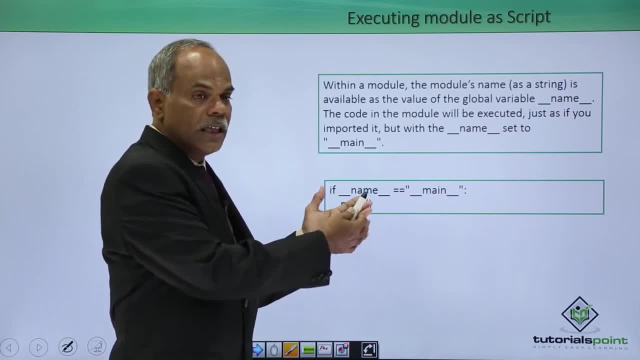 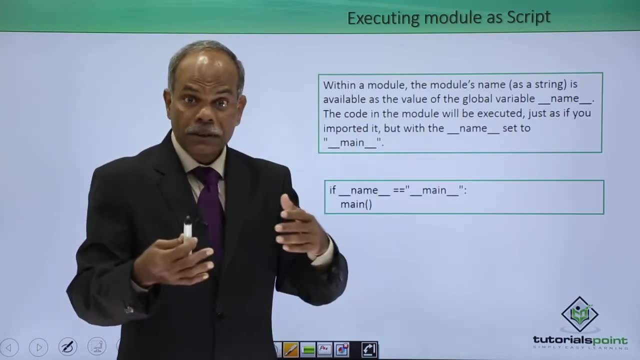 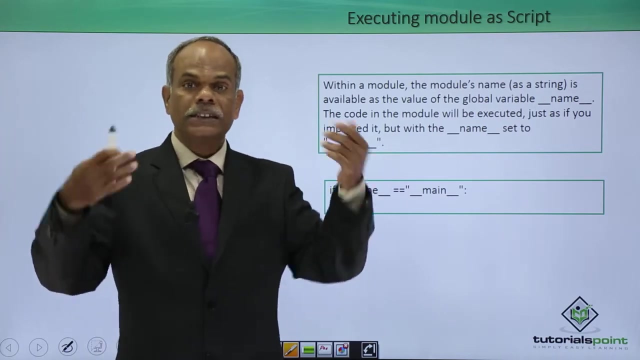 So how this is done. In order to show this, I have an example in which this syntax is used. The script is that script is. you know, it is possible to include that script in another and it is possible to run that script itself. How it is done. 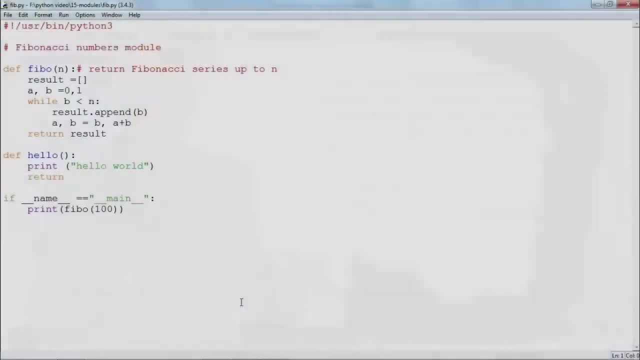 We will demonstrate this by running that example in front of you. Python interpreter is able to Understand whether a particular Python script is being used as an import or if it is being used as a executable script. That is done by the value of the global variable called underscore- name- underscore. 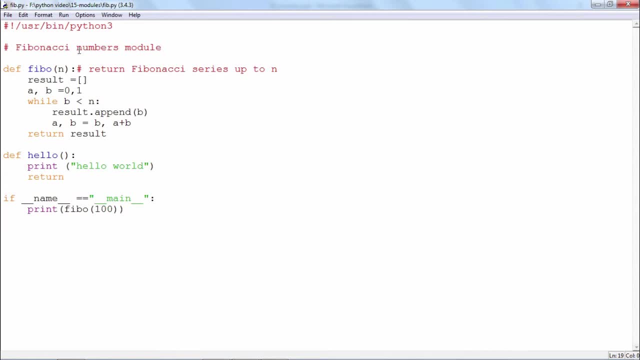 If this Python script is directly run, Then the name, The value of this Global variable Name, is equal to main. On the other hand, if this script is imported into another Python script, then, As far as this model is concerned, the value of the variable name is not equal to me. 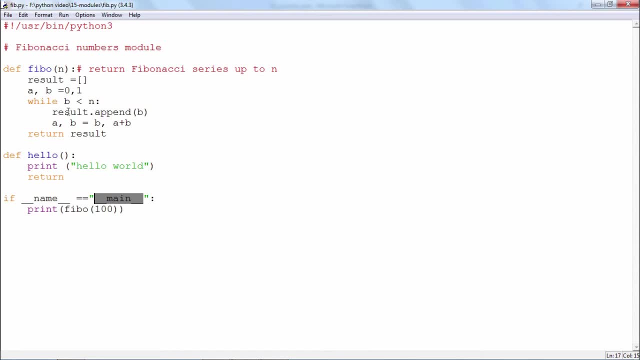 So if I run this, then For this Python script, then value of the global variable underscore- name underscore- will be equal to main. So you can, You know, Treat this As the main function in your Executable Python, Similar to what we see in our C or C++ program, where the entry point of your program is main. 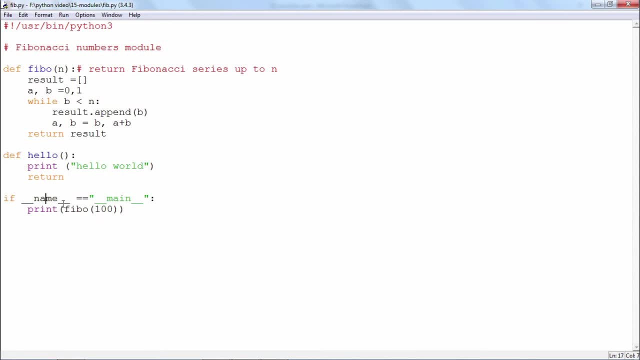 Right. So if I run this, This is my main function, And from the main function I am calling this Fibo function, which will generate the Fibonacci series up to 100.. So a module can also be Used As an executable script. 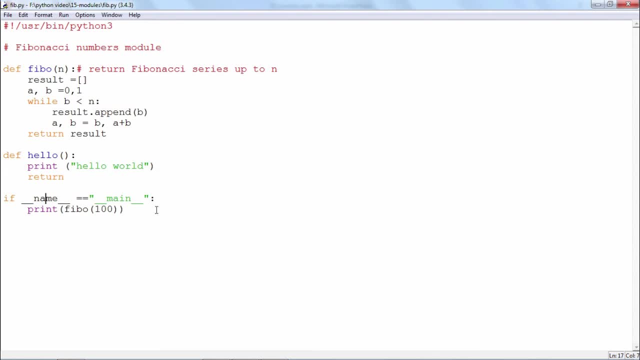 Identify whether that module is being Used as an executable script or not Can be, Can be, You know, Found out by This statement. If this is true, then Whatever you want to Execute from the main can be done.